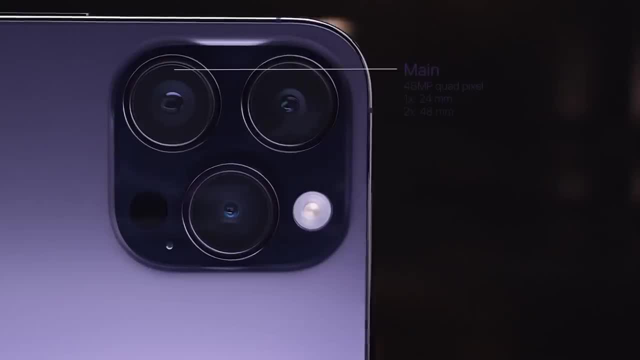 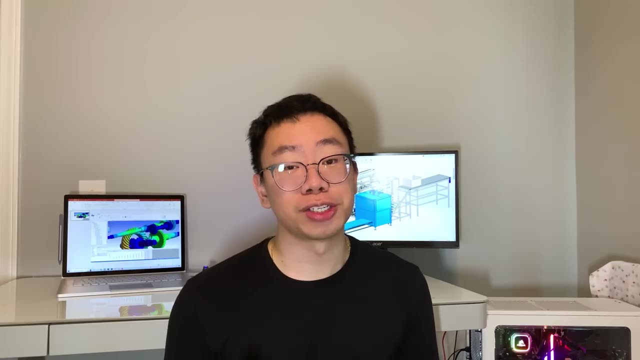 the phone must offer, such as dynamic island, and how many lenses the camera has to have. They'll also tell us that it must be splash, dust and water resistant. To start out, industrial or product designers will create a digital surface model that details what the product will look and. 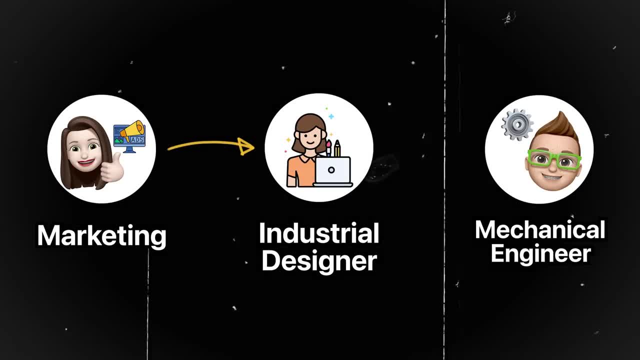 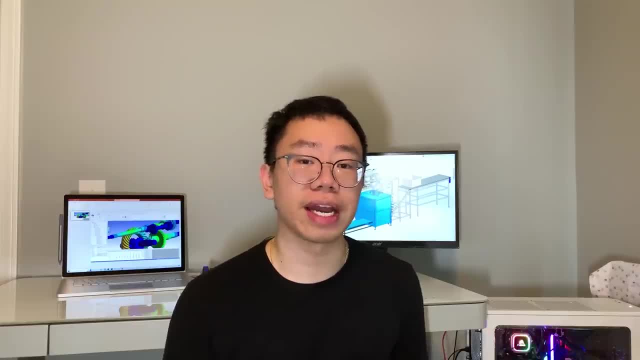 as a step file, so that we can import it into our computer-aided design or CAD software, such as Inventor, SOLIDWORKS, Creo, NX or CATIA. This way, we know precisely how much space we have to work. 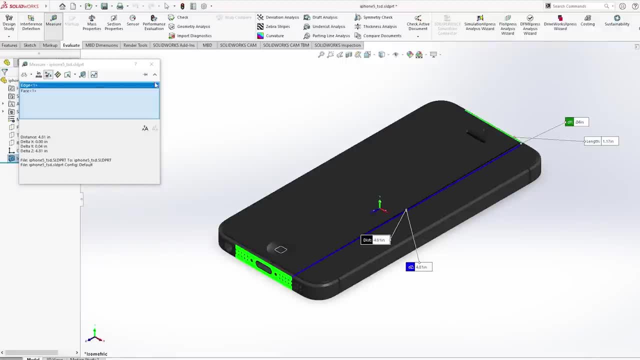 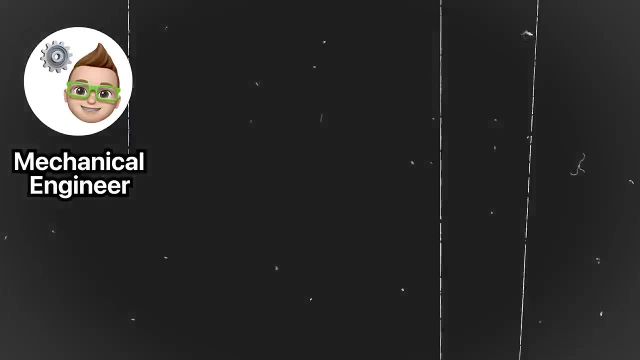 with, and how big or small, to make internal components. Next is the second step: prototype design. Here we will work with other mechanical engineers in the same team, as well as electrical manufacturing, optical and software engineers, to create a proof of concept that demonstrates the 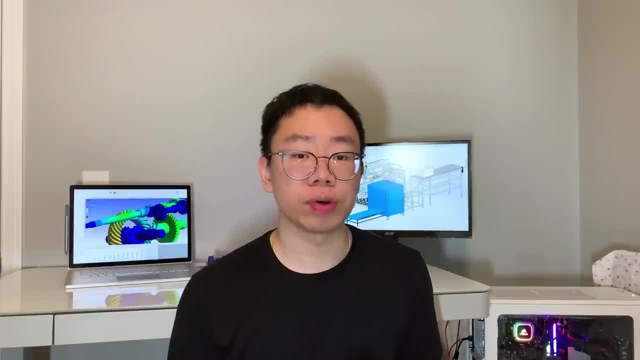 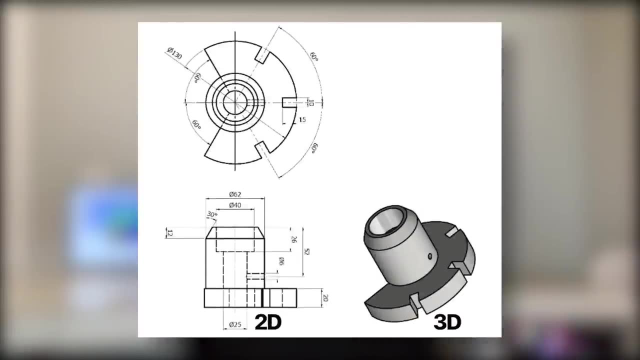 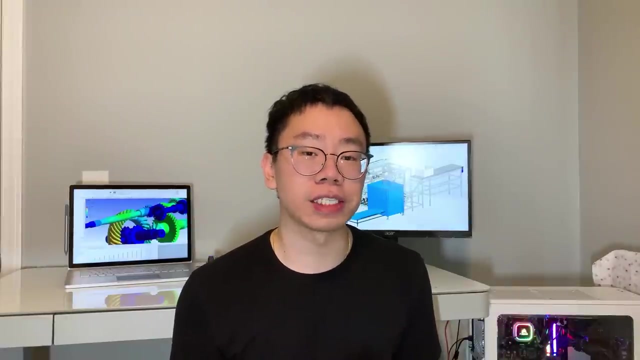 product's basic features and feasibility. In this stage we will use CAD software, say SOLIDWORKS, to create high-level preliminary 3D models of each component and corresponding 2D technical drawings so that each part can be made later on. However, keep in mind that the manufacturing processes used 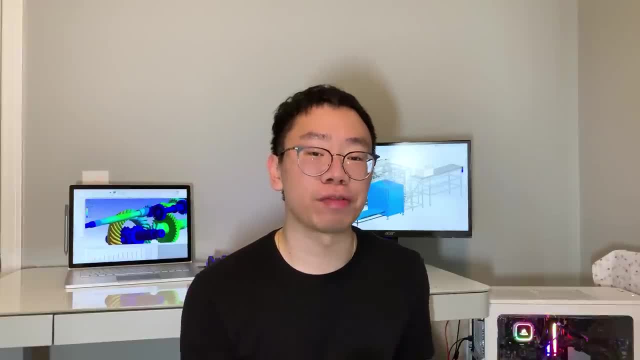 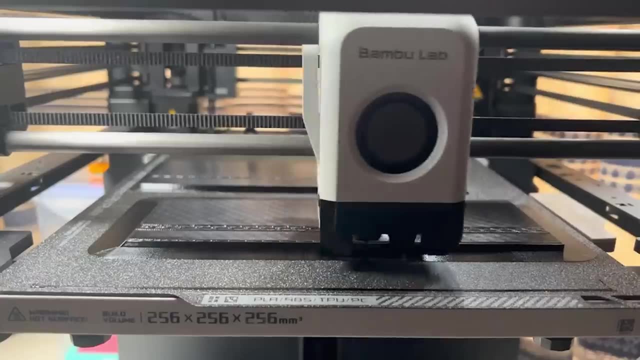 to make the parts of the proof of concept will ultimately differ from the processes used to make the parts of the final product. for example, let's say we're designing a phone. we would use 3d printing to create multiple iterations of the phone's chassis for the proof of concept and in 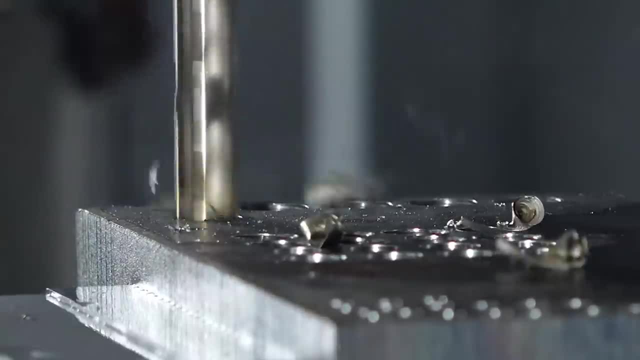 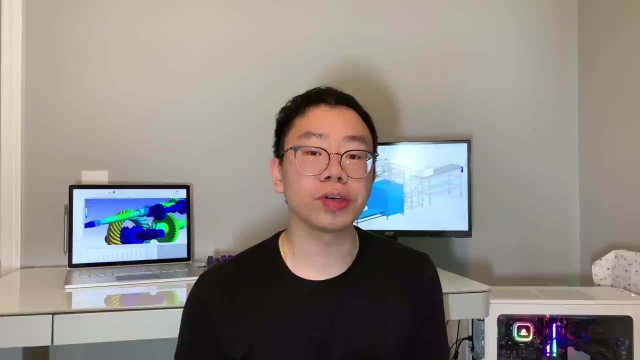 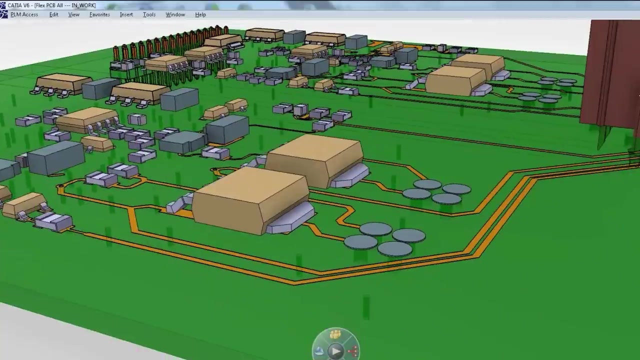 the next stage we refine the part design so that it can be mass produced using cnc machining or casting in a cost effective and efficient way. we will also begin to gather initial information from electrical and optical engineers to see how big the printed circuit boards, sensors, battery. 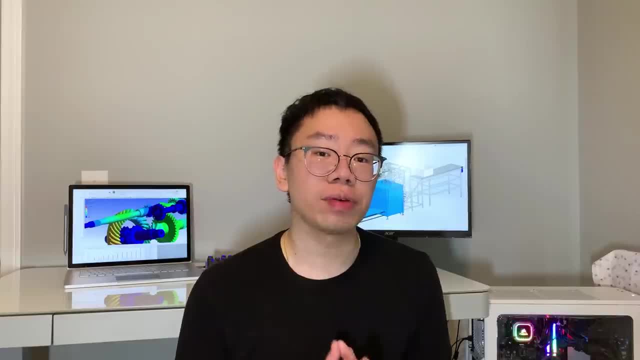 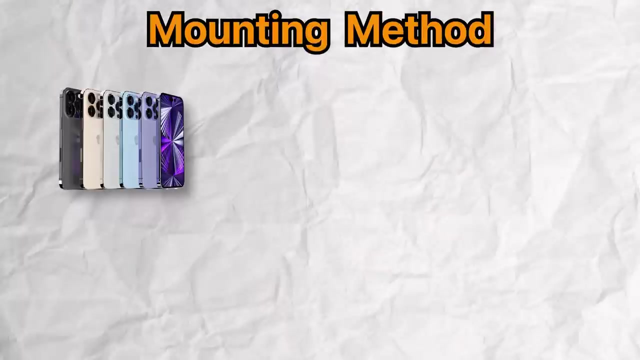 camera lenses and wiring need to be, and how everything will fit together, be mounted and sealed. obviously, the design will constantly evolve and change as we move through the product development process and all aspects of the design is fine-tuned. for example, in the final product, the internal electrical components will be secured via mounting features, such as screw bosses, using a 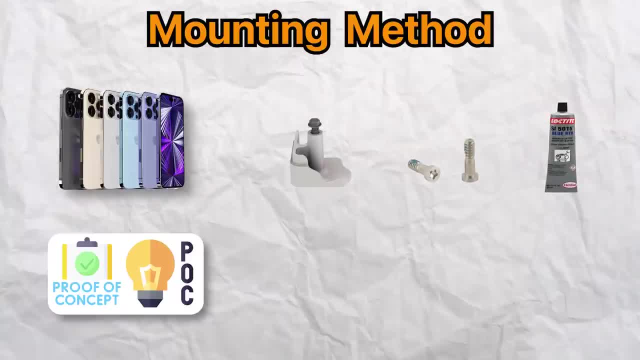 combination of screws and special adhesive. but for the proof of concept, these mounting features would not be included in the final product, so we will continue to work on the final product. and we will continue to work on the final product. so we will continue to work on the final product. 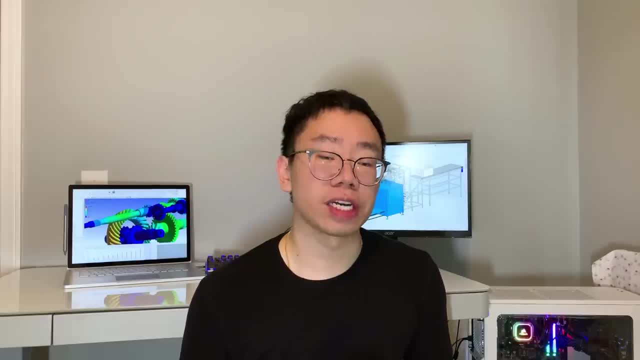 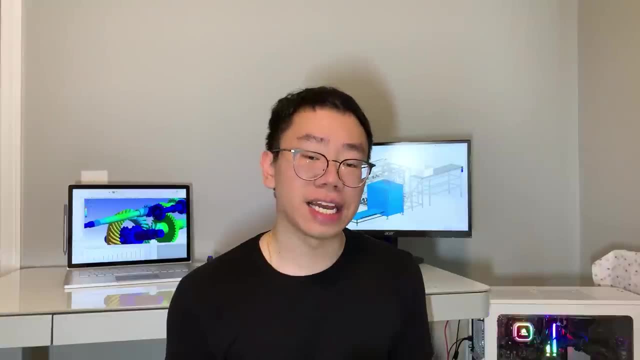 and double-sided tape will be used instead. many features and components like buttons and side switches will be replaced by dummy components in the proof of concept. in this stage we will also begin selecting materials for each component based on functional and technical specifications of the product. for example, if the phone's chassis needs to be corrosion resistant, dissipate heat quickly. 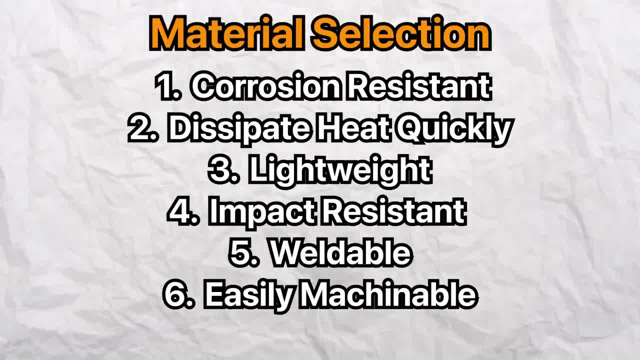 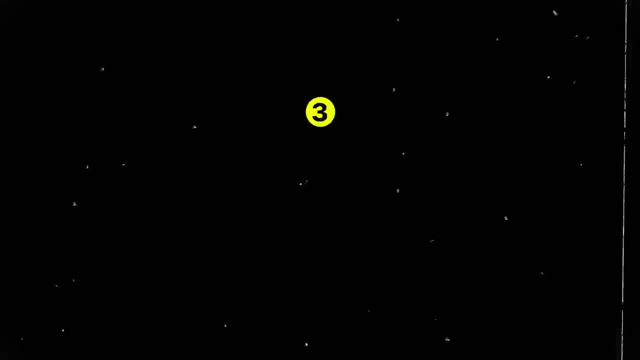 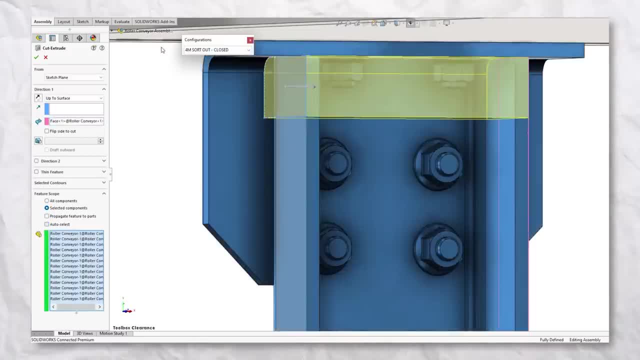 lightweight, impact resistant, weldable and easily machinable, then we would need to use a systematic method to choose the optimal material, such as an ash beecher. moving on to the third step, we have detailed design. this is a very critical step where we design and incorporate all of the 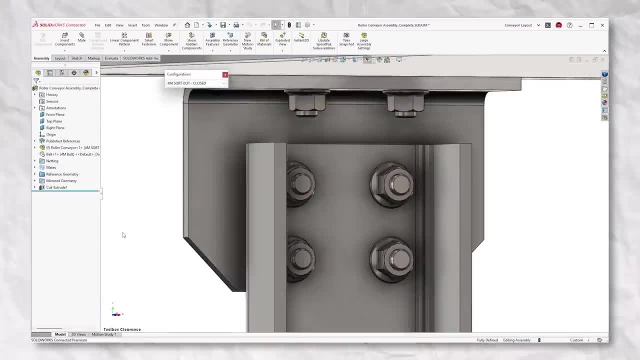 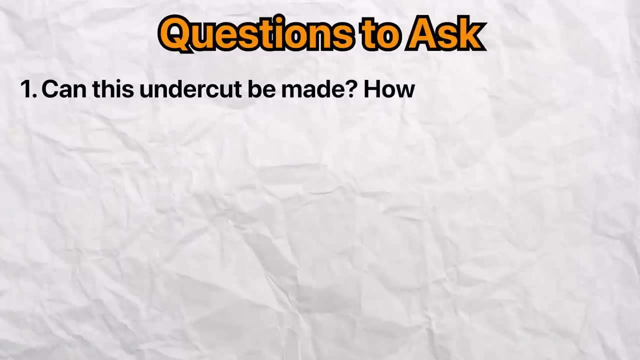 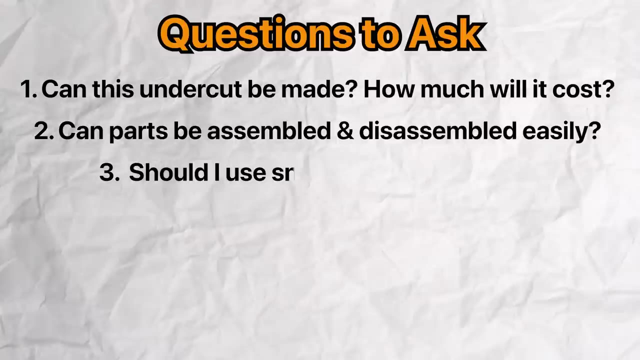 mechanical features of the actual product into the 3d cad model for each component and sub-assembly. you need to ask questions like: can this undercut be produced? if yes, will it drive up part cost? can these parts be assembled and disassembled easily? can we use snap features or screws to mount this part? does this part require a loose or tight tolerance? 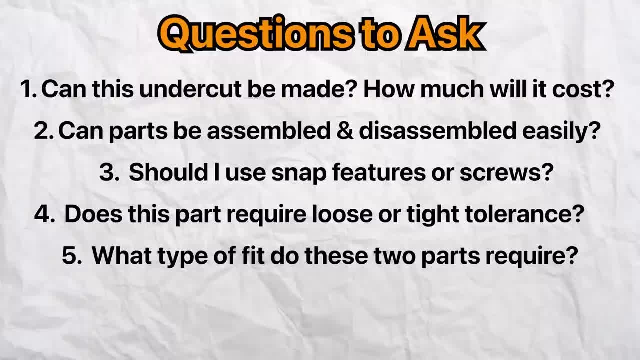 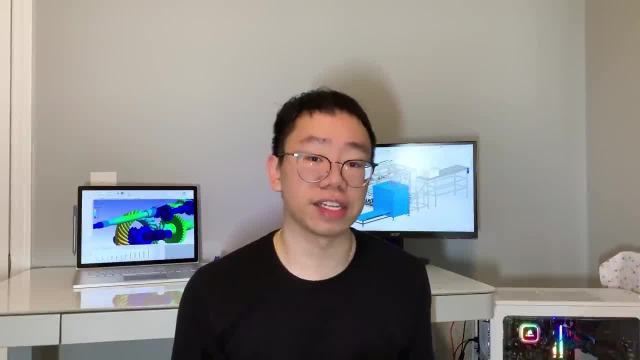 do these two parts require a clearance, transition or interference fit. once the design is pretty much nailed down, we create and release the production drawings, which look like this: these drawings show different views of the component and call out critical dimensions, tolerances and specify information about the component's material. 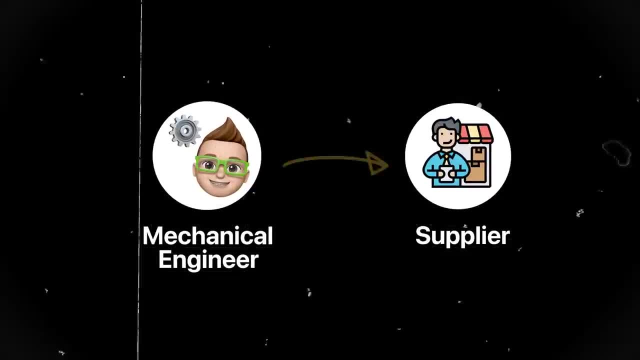 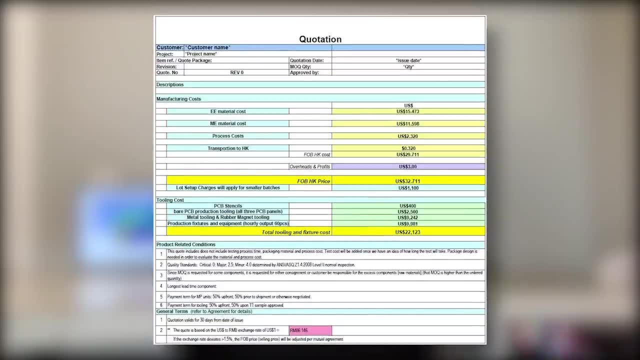 surface finish revision number. we then send these drawings to different suppliers, who give us valuable manufacturing feedback as well as a quote which details the total cost needed to make, assemble and ship these parts. we will also create a bill of materials or bomb, which is just a list containing. 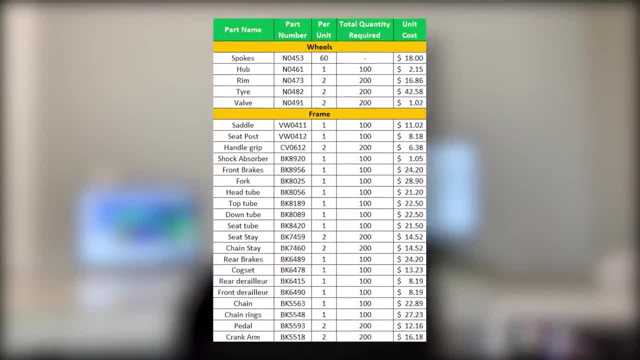 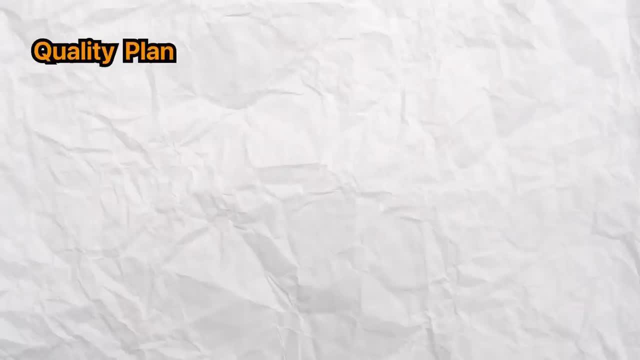 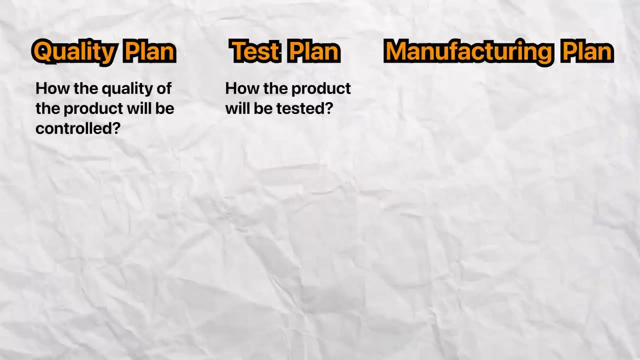 all of the parts, sub assemblies, their part numbers and quantities of each needed to make the final product. we will also work with quality and manufacturing engineers to create the quality test and manufacturing plans explaining how the quality of the product will be controlled, how the product will be tested, and what processes, equipment and how much labor will be required to assemble. 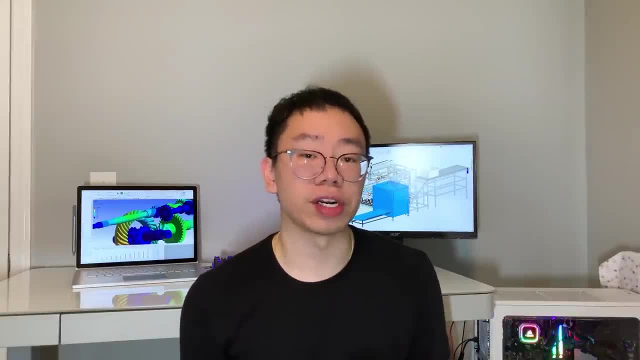 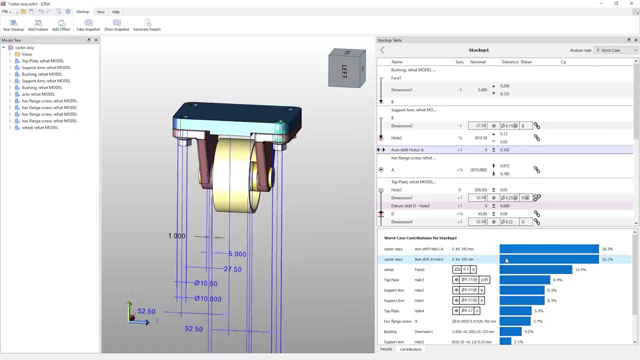 the final product. in this stage, electrical and optical engineers also need to provide us with the finalized printed circuit board layouts and optical designs containing important information such as sensor location, so that we can begin to finalize the cad model and perform a tolerance stack up analysis to make sure that everything fits together and that there are no interference issues. the entire 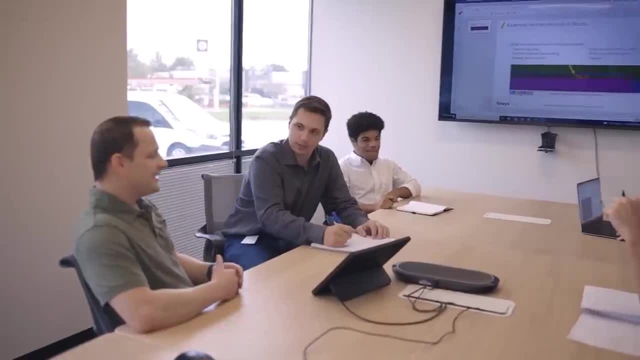 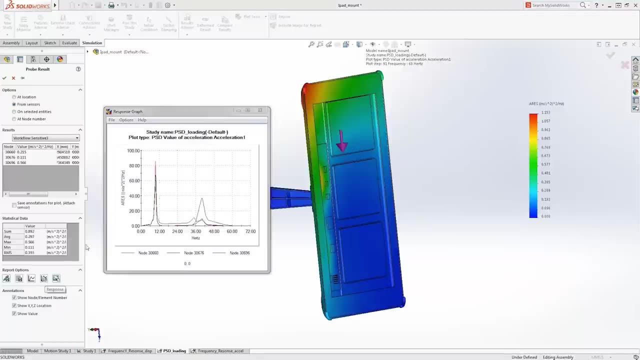 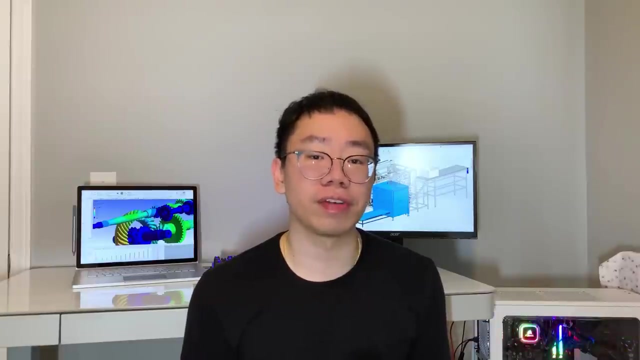 engineering team will have several technical design reviews to identify weaknesses in the design, potential failures that might occur, such as battery leakage, and the effects of these failures before the product is actually manufactured, assembled and sold. a common approach used in industry for identifying failures, causes and effects is fair modes and effects analysis, or fmea. 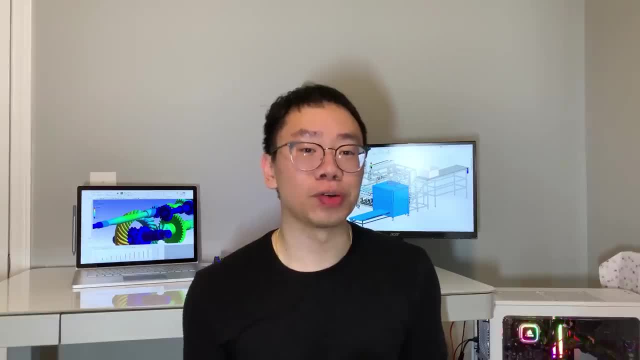 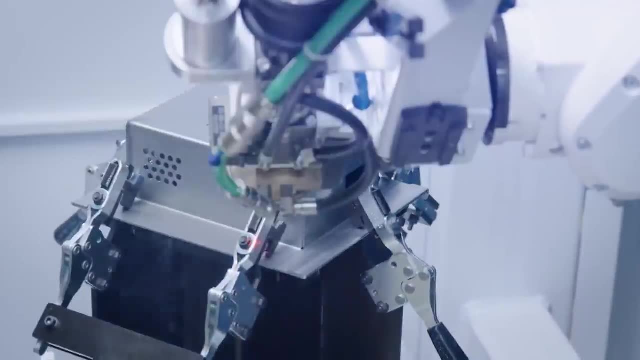 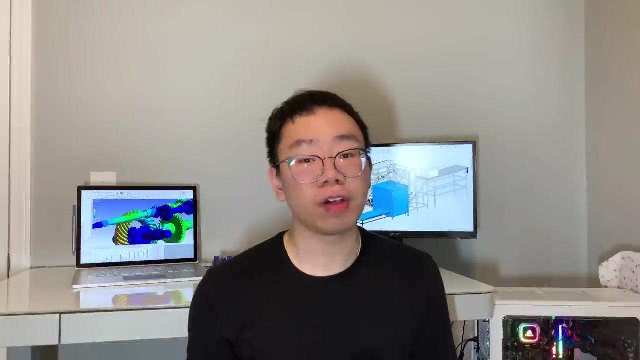 which most schools don't teach. finally, the last thing we do is source parts to build 20 to 50 units, using the intended materials and manufacturing processes for engineering, design validation, testing or evt, to ensure all functional product requirements are met if, say, a design flaw is discovered during. 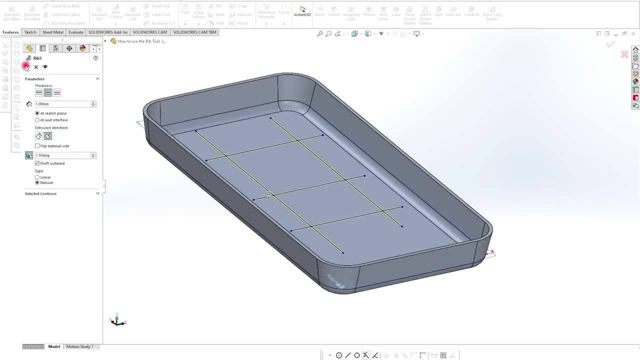 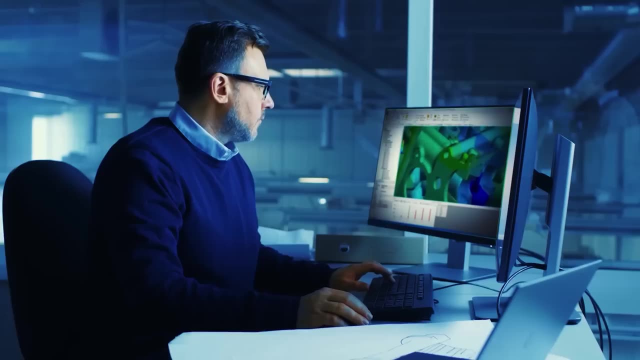 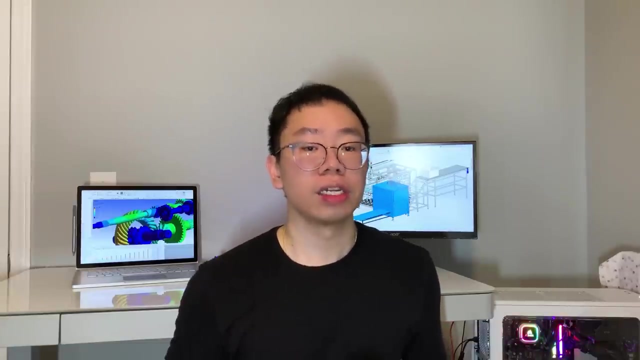 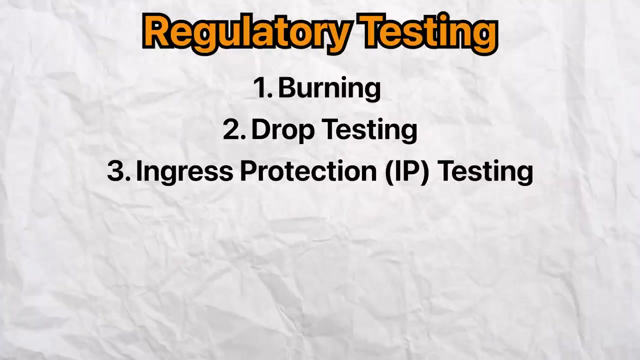 testing, we will go back to the drawing board, improve the design by adding structural ribs and then run a finite element analysis study to validate the performance of the design change. we then move into the validation stage. this stage focuses on testing the out of the product. typically we send 50 to 200 units for rigorous regulatory testing, such as burning drop testing. 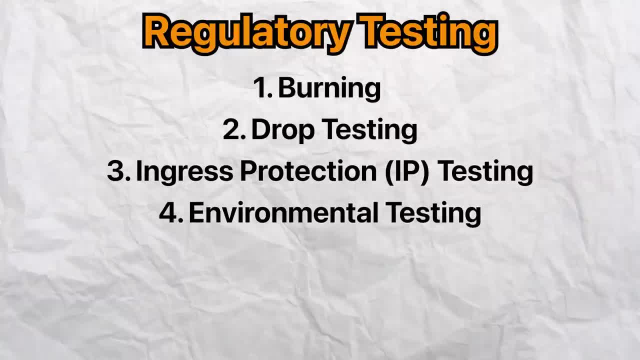 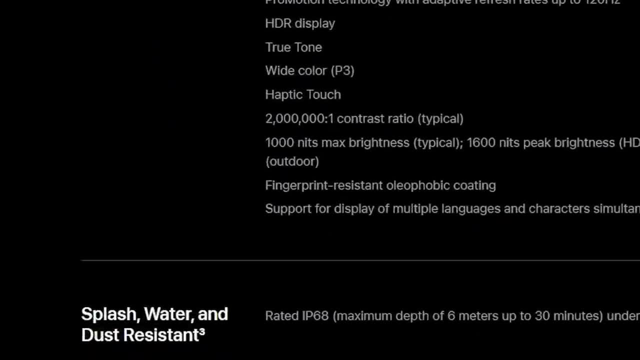 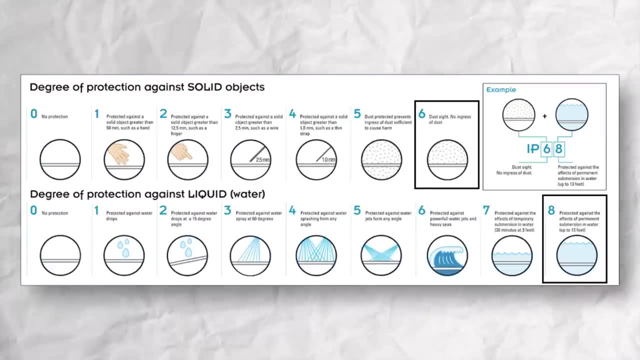 ingress protection testing, environmental testing and extensive battery testing. take an iphone 14, for instance. apple advertises that it has an ip68 rating under iec standard 60529, which just means that this phone is water resistant up to a depth of 6 meters for 30 minutes in order to receive. 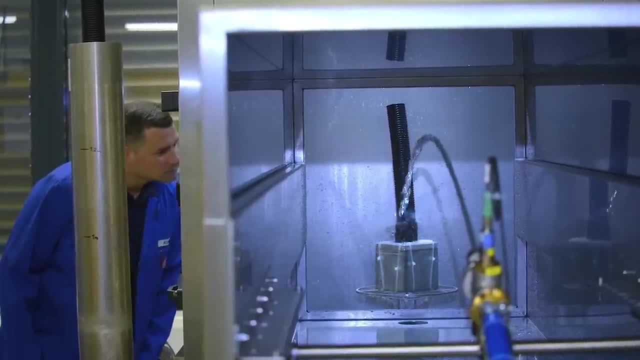 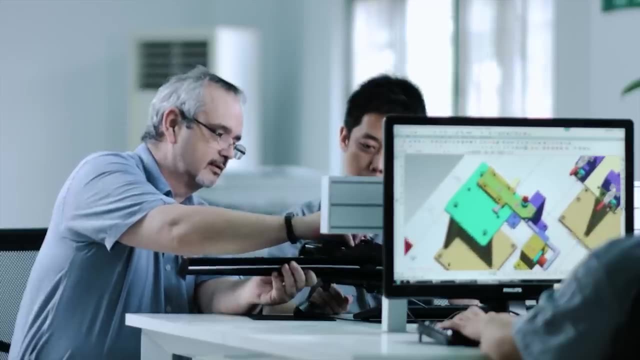 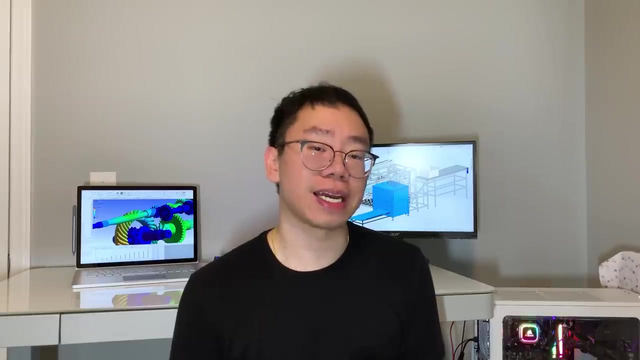 this rating. apple probably had a certified tesla performed the ingress protection test. for smaller companies, you might also be responsible for designing fixtures used to test the product or fixtures and jigs used to hold components in place during assembly of the final product. larger companies like apple will partner with contract manufacturers like foxconn, who does. 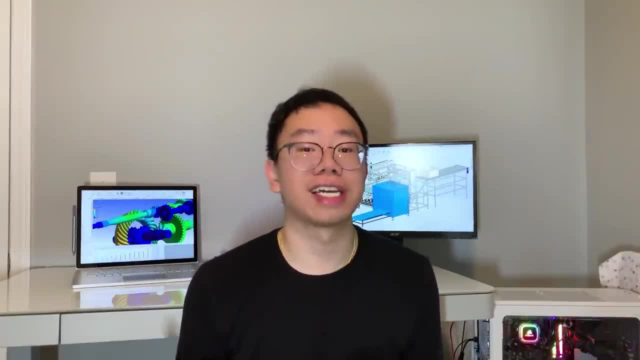 everything for them. after putting the product into the computer interface application, use the operating system to create auel скорее phone or camera device feature. so apple will not be able to run manuals or gear system integration. the product through so much testing, we move into the optimization or refinement stage. in this stage it's 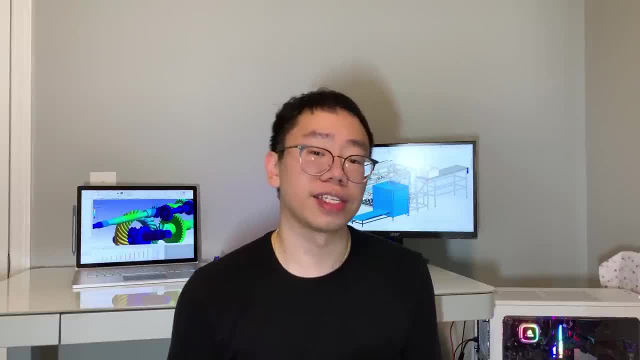 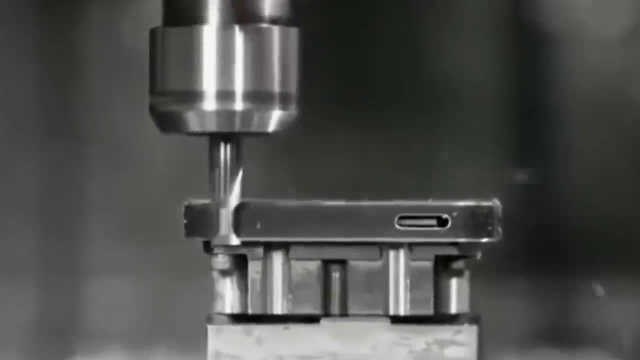 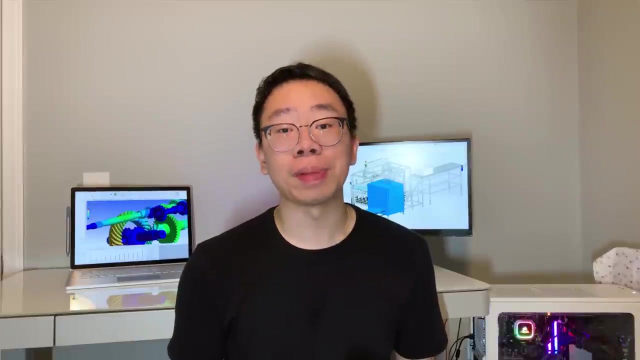 very likely you'll find some weak points in the product, whether it's design, quality or manufacturing related. this is the last opportunity for you to figure things out and get things right before the product is mass produced and sold. we'll also work with manufacturers to ensure that manufacturing. 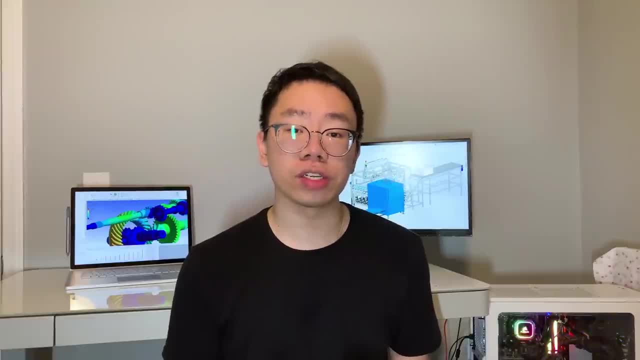 processes such as tooling are fine-tuned, quality assurance and control procedures are finalized so that high quality parts are coming off the line and any outstanding issues like packaging is addressed. the design becomes frozen at this stage, which simply means that any subsequent engineering change that needs to be made will require us to first complete an engineering 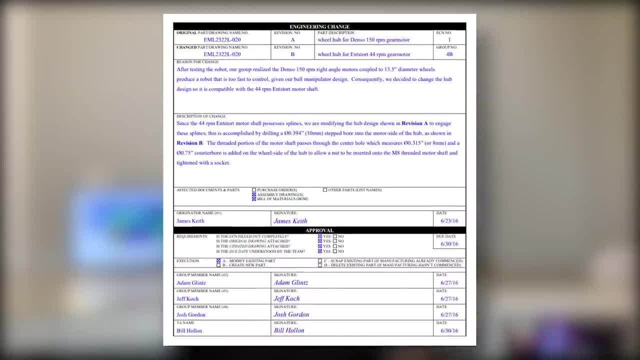 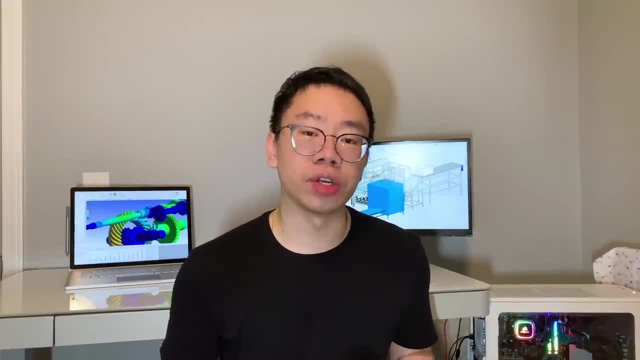 change notice, or ecn, whose purpose is to document the design change and the reason for the change. for example, if i were to leave the company and two years later a new engineer was working on the same product, he or she could see all the design changes that were made and when exactly they were. 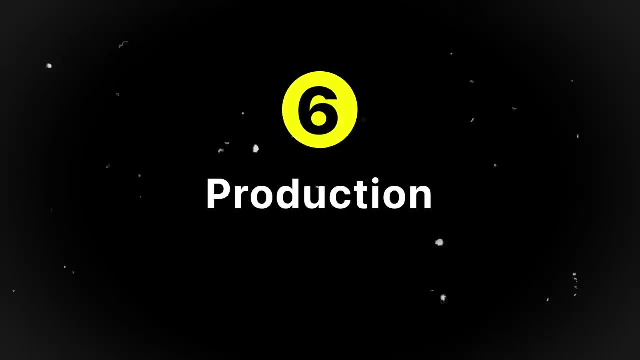 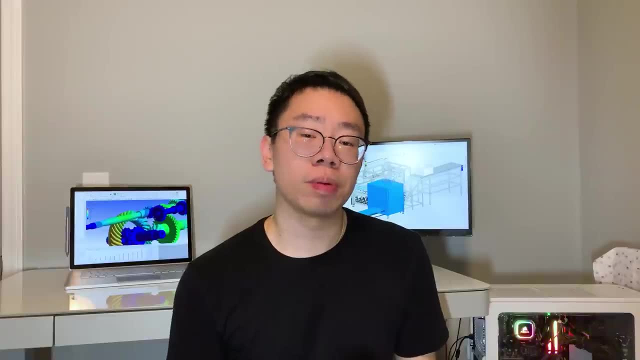 made. finally, the last stage is production, and at this point mechanical engineers are usually completely hands-off. some minor issues that require your support might come up from time to time, but it's very likely you'll already be assigned to a new project by your engineering manager. all of the things i mentioned so far are 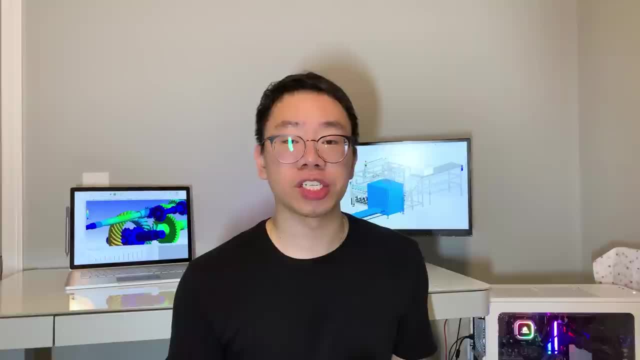 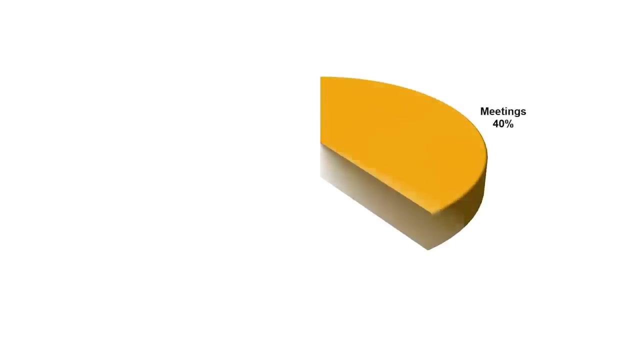 engineering related, but keep in mind that almost every engineering job will come with a lot of non-technical and administrative duties, which i like to call busy work. if i had to break down the time i spend doing all the different types of work as a mechanical engineer, i'd say 40 of my. 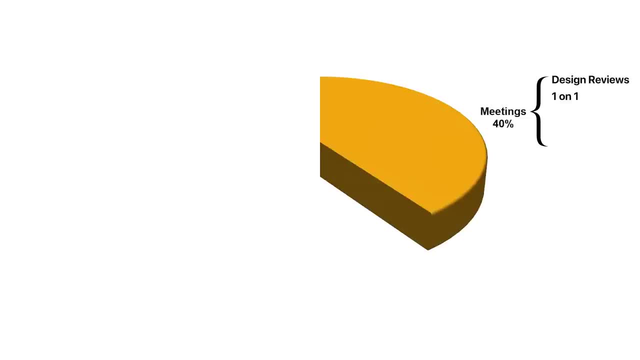 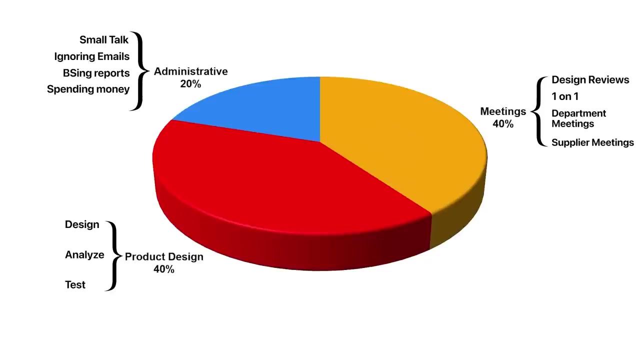 time is spent in meetings, which includes design reviews, one-on-one meetings, department meetings and meetings with suppliers. forty percent is spent designing, analyzing or testing products. finally, the remaining 20 is spent talking to people, replying to emails, writing reports, ordering parts or raw materials and completing engineering change notices. obviously, every mechanical engineering.